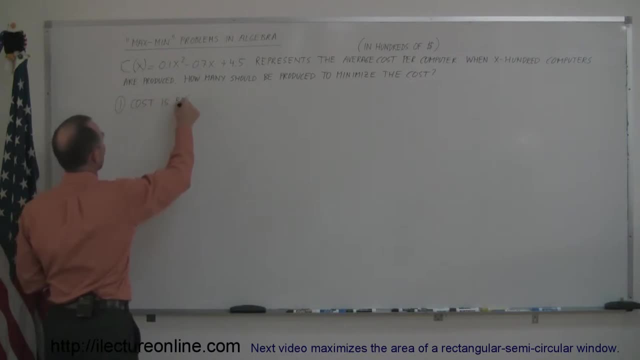 We get that the fundamental Everyday Cost is being minimized. so always determine what's being maximized and minimized. Okay, the second thing you always do is try to find an equation representing the item that's being maximized or minimized. In this case it is the cost. so cost as a function of X is equal to 0.1 X squared minus 0.7, X plus 4.5.. 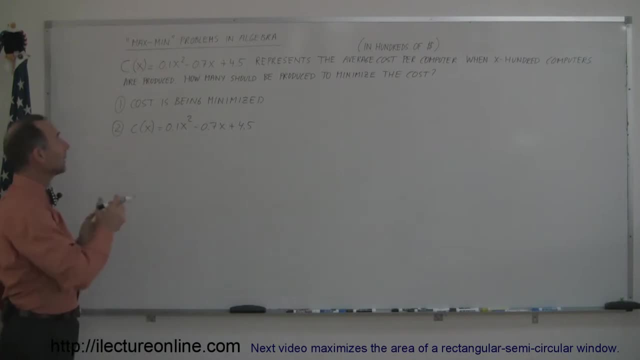 in this case, We don't have to go and eliminate any variables, because C is written in only one variable, which is great, So we don't have to find any constraint. That's really good. The next thing to do is to realize that we're dealing with a quadratic equation. 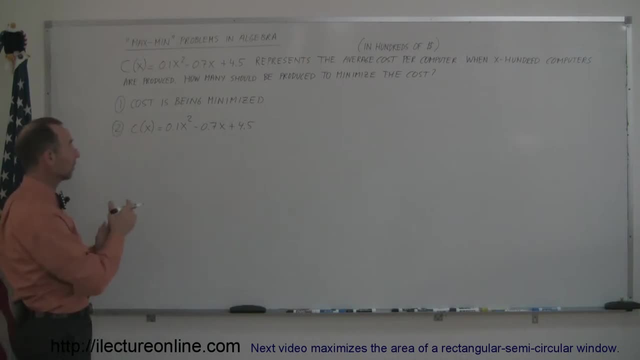 which is represented by a parabola. if we draw this graphically, And since the x squared term is a positive, we can then see that the parabola will open upward like this, And it'll be somewhere on the xy axis, doesn't matter where. we just have to realize it opens upward. 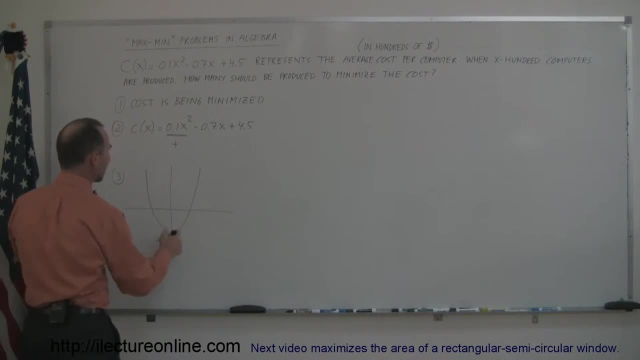 which means that there'll be a place, somewhere, where the minimum value of the parabola can be found, And that would be x sub v, y sub v, meaning x and y, or in this case not y, but c, are the vertex, or the coordinates of the vertex of the parabola. 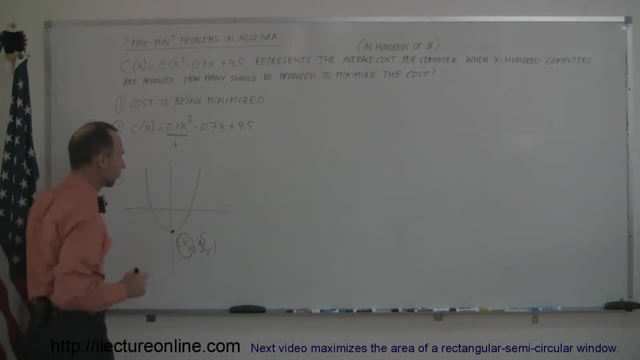 And what we're trying to find is the x coordinate of the vertex. in this case, And if we remember right, the equation to find the vertex of the parabola is the vertex of the x value or the x coordinate of the vertex, I should say x sub v. 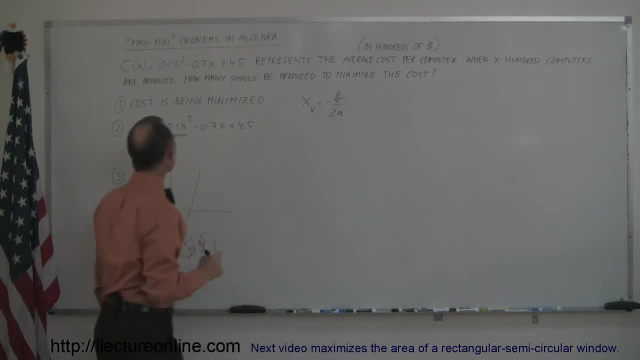 that's equal to minus b over 2a, realizing that a is the coefficient of the x squared term, b is the coefficient of the middle term and c is the coefficient of the constant. but of course we don't need the c in this particular case. 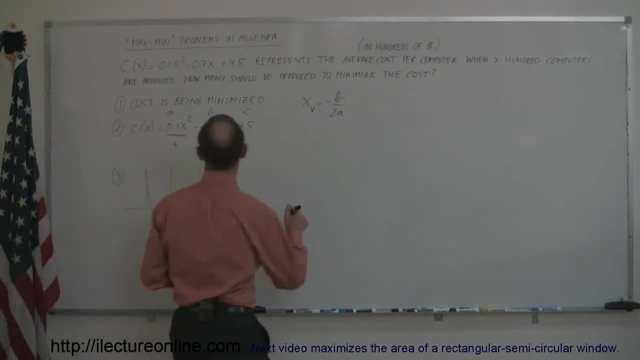 All right, now plugging in what a and b are equal to: a is equal to 0.1,, b is equal to minus 0.7, so x sub v is equal to minus times the minus 0.7,. 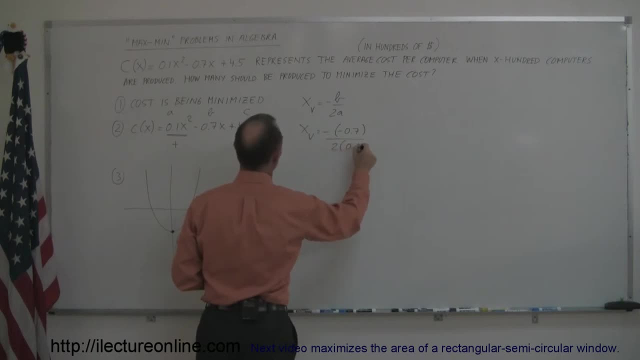 divided by 2 times a, which is 0.1, so x sub v is equal to 0.7 over 0.2, and so x sub v is equal to 3.5.. So what that means is when x is 3.5,. 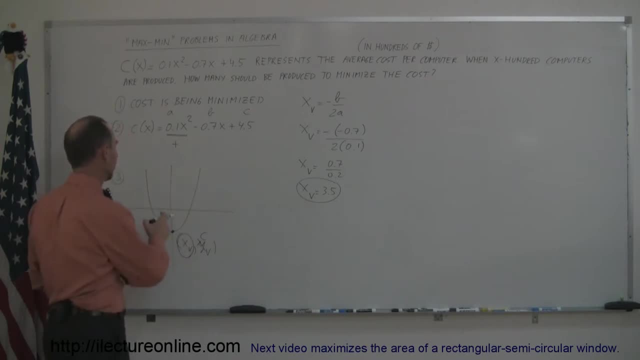 and of course, x is hundreds of computers. we should have minimum cost. So therefore, we can say that we need to build 50 computers, and what will then be the minimum cost? Well, we can then plug in the value for x in the cost function. 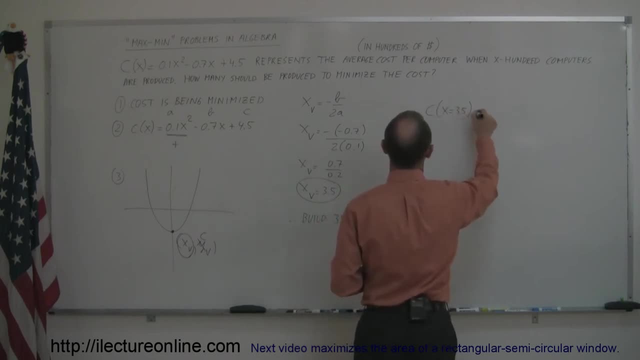 so c, when x is equal to 3.5, is equal to 0.1 times 3.5, squared minus 0.7 times 3.5, and then plus 4.5.. All right, let's work that out. 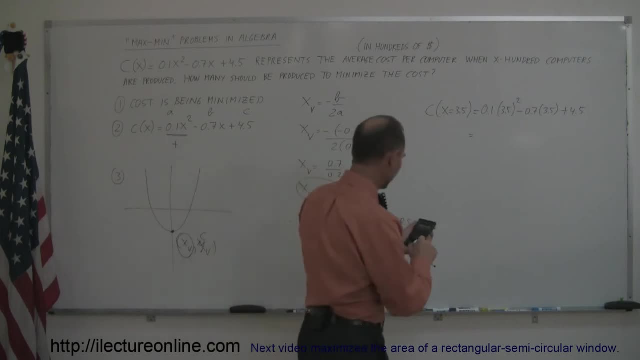 I think I'm going to grab a calculator to do that. So we have 3.5 squared. we multiply that times 0.1,. we subtract from that 7 times, or 0.7 times 3.5,. 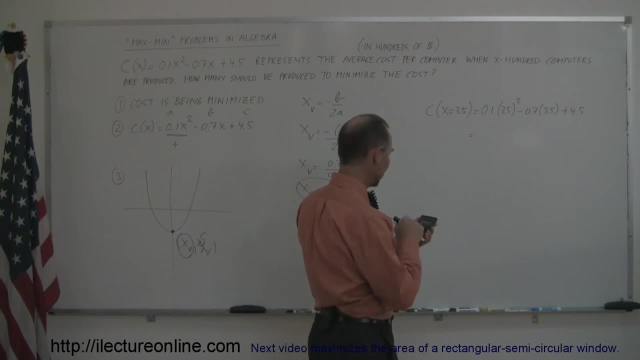 0.7 times 3.5, and then we add to that plus 4.5.. Equals, and so the cost, when x is equal to 3.5, is equal to 3.5, is equal to 3.275,. 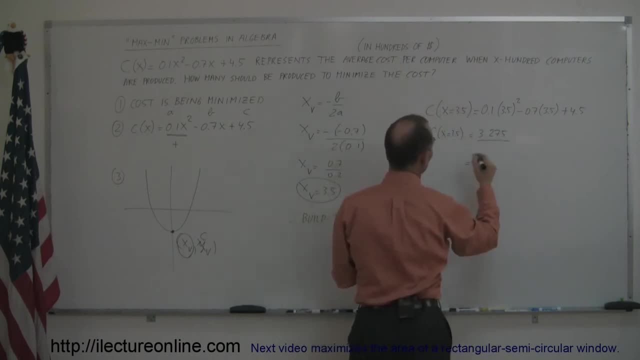 which is in hundreds of dollars. so therefore the minimum cost is $327.5, when our production run makes 350 computers and I guess this is a per day production or something like that. So to maximize profit you want to minimize cost. to have minimum cost. you want to build 350 computers a day. your cost will be $327.50 per computer. Notice that if you only build, if you build zero computers, your cost will be $450 per computer, although that does make a lot of sense. 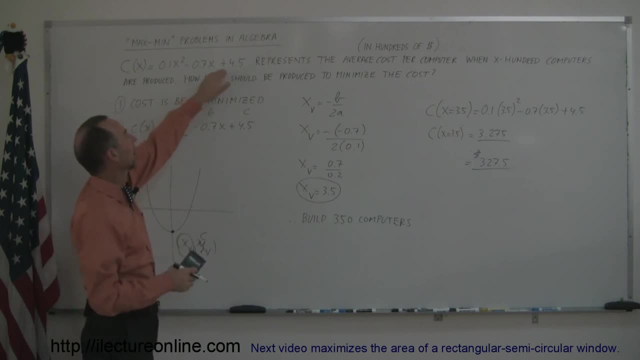 You can see that there's some initial cost to keep the shop running and that will then be negated by building more and more computers. I would then assume that if you build too many computers then it becomes very inefficient and the cost per computer will go back up. 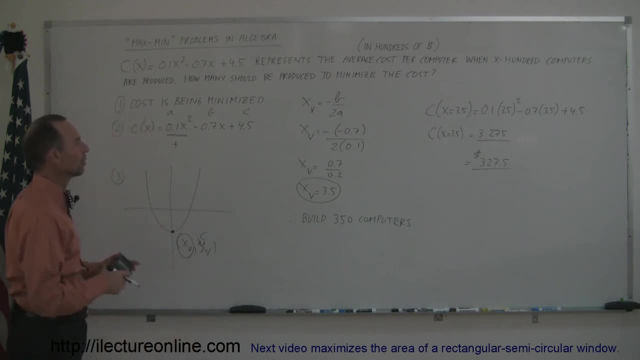 That's kind of like an industrial equation or an equation that we can use in an industrial setting where we're building or manufacturing something, and it's a very useful way to look at manufacturing costs. All right, so hopefully this helps you, and let me see if I can think of one more example. of how to work with max-min problems in algebra.